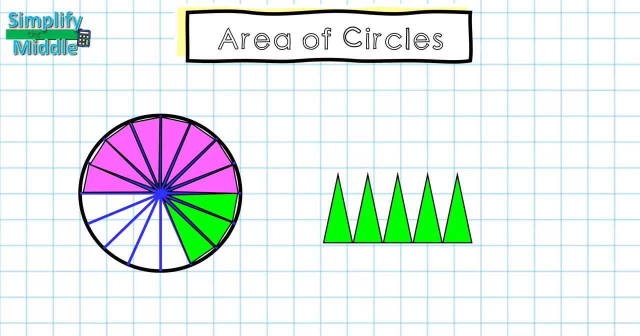 I'm going to go ahead and pull out the bottom half of my circle and I'm going to align them into a straight line here. Now, remember, this is the close approximation, because it is flat instead of curved on the bottom. But if I was to look at the distance from here to here, that would be about half the circumference, because we know that it's on the outside edge and it's inside the circle and it was only the bottom section. 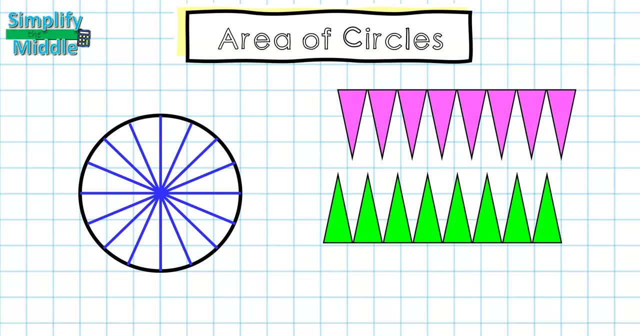 So when I take out the pink section, I'm going to align those as well. But something interesting happens: when I place them together, It creates what looks like a parallelogram, And this is going to help us for understanding where the formula for the area of a circle came from. We know the area of a parallelogram is going to be length times height. It's very similar to the area of a rectangle, but instead of length times width, it's length times height, Because we can't use this diagonal piece. 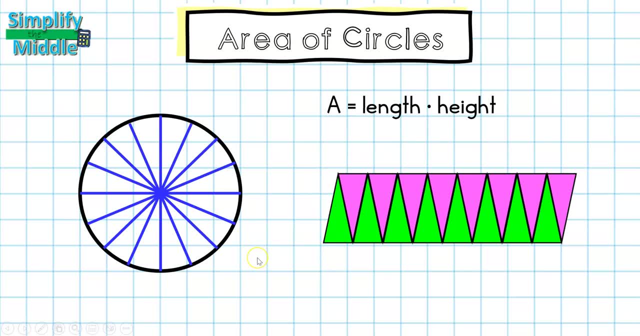 So we need to find the measure from here to here. Looking at the circle, there's something interesting: The distance from the center to the outside edge happens to be the same distance from the bottom to the top of this parallelogram, And that distance in this particular circle is our radius. So I'm going to replace that line with the letter R for radius. We already said the distance from here to here is half the circumference, And we know there's two circumference formulas. 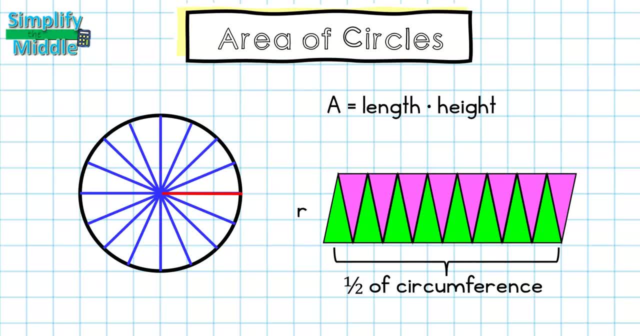 There is pi times diameter or two times pi times radius. So I'm going to use that formula and I'm going to place it over two to represent the half of the circumference. So here's the circumference formula and here's half of it. When I do that, I notice that two divided by itself is going to be one. So those actually cancel out. 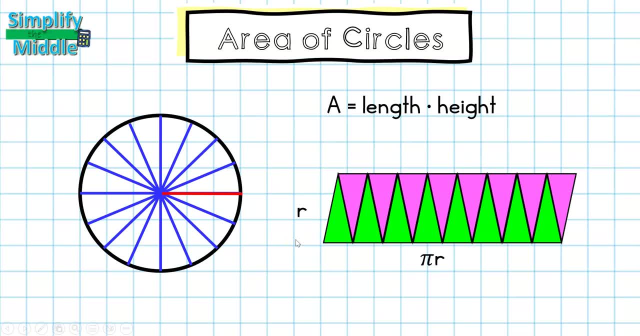 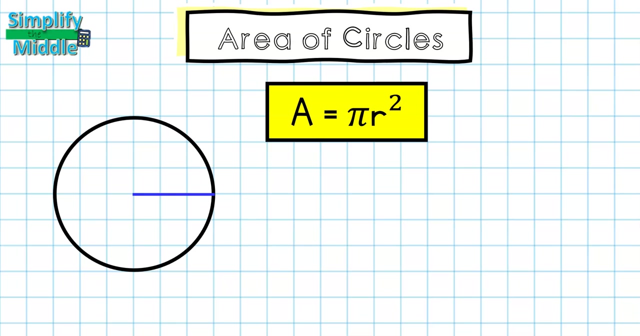 Then I'm left with dimensions that this parallelogram is radius and height and pi times radius and height And length. So I'm going to multiply all three of those together And I end up with area equals pi times radius, which is the length of my parallelogram times radius for the height, or area equals pi times R squared. Now that we have our formula, let's go ahead and apply it. So the first step of solving any circle problem is to go ahead, for our area is to go ahead and rewrite the formula. So I'm going to write: 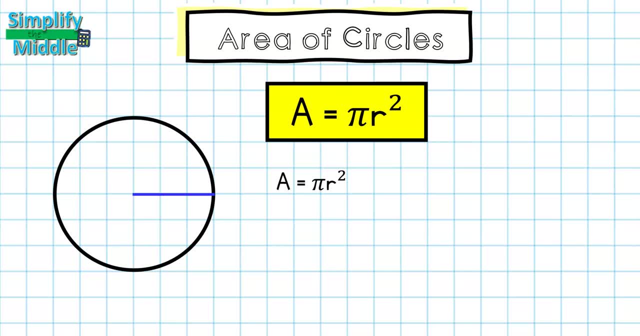 area equals pi times R squared. Something important to think about here is that this is not radius times two, So I don't get this confused. I'm going to rewrite this as area equals pi times radius, times radius. This just helps me remember that I'm going to be multiplying the radius by itself here. The next part is to find out what is the radius in this circle. They did not tell us the dimension, but they 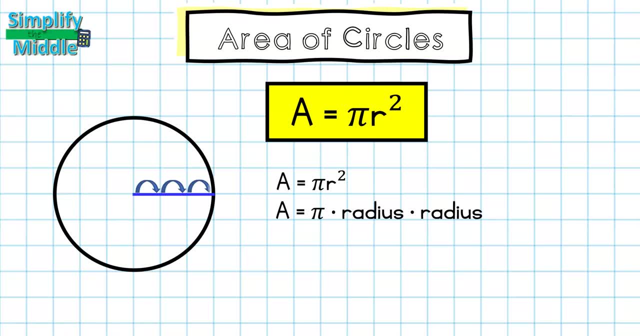 do have it on grid paper so I can count. So I can see that it has a distance of three. So this radius is three units. Now I'm ready to substitute in my formula, So I'm going to be using 3.14 as an approximation for pi, So I have area equals 3.14 times three, times three, because I will be writing my radius twice And my last step is to multiply. So area is approximately 28 and 26. 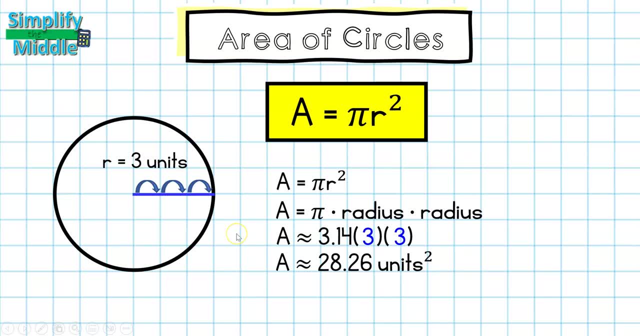 hundredths units squared. In my circumference problems I was talking about one dimension, But in this I'm talking about two dimensions because I'm talking about the area inside, So I have to write my units squared. Let's look at another example. Here we have a circle that is 16 feet by diameter, So let's go ahead first and write out our formula: area equals pi R squared, And I always like to rewrite it, So I'm going to rewrite it.